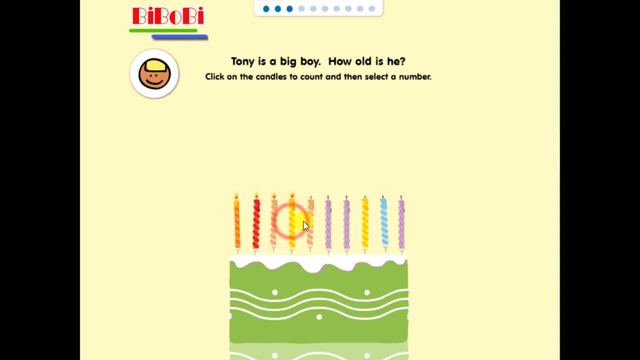 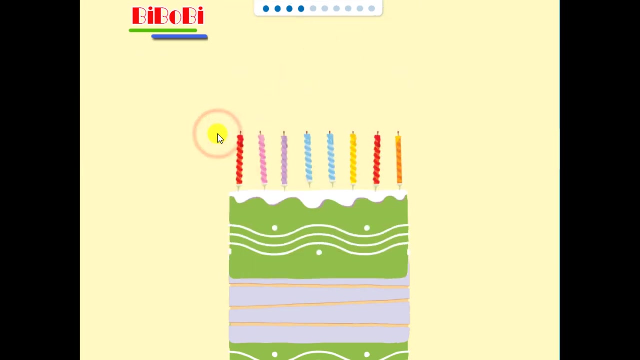 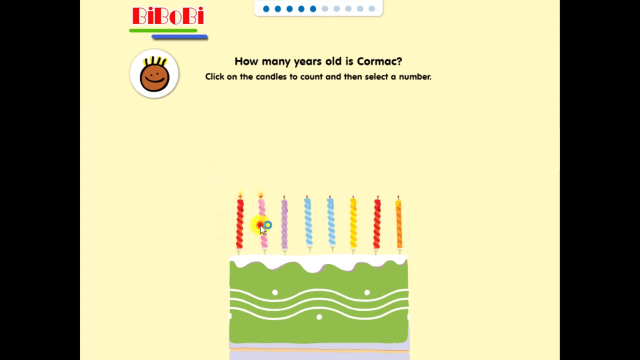 One, Two, Three, Four, Five, Six, Seven, Eight, Nine, Ten, That's right. How many years old is Alan? One, Two, Three, That's right. How many years old is Cormac? One, Two, Three, Four, Five, Six, Seven, Eight. 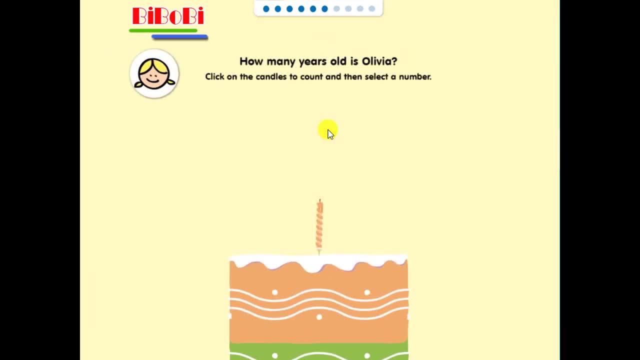 That's right. How many years old is Olivia? One, That's right. How old is Noah? One, Two, Three, Four, Five, Six. One Two, Three, Four, Five, Six, Seven, Eight, Nine One. 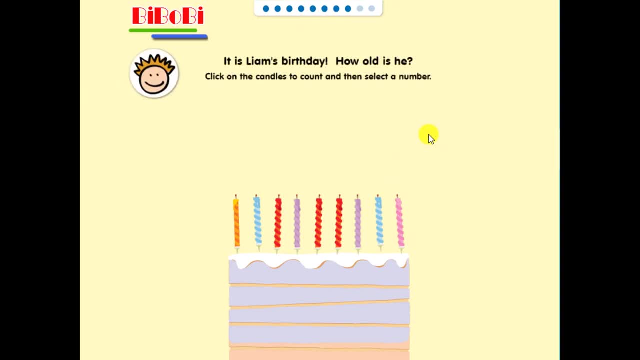 One, Two, Three, Four, Five, Six, Seven, Eight, Nine. One, That's right, It is Liam's birthday. How old is he? One, Two, Three, Four, Five, Six, Seven, Eight, Nine, Ten, Eleven Men years old. 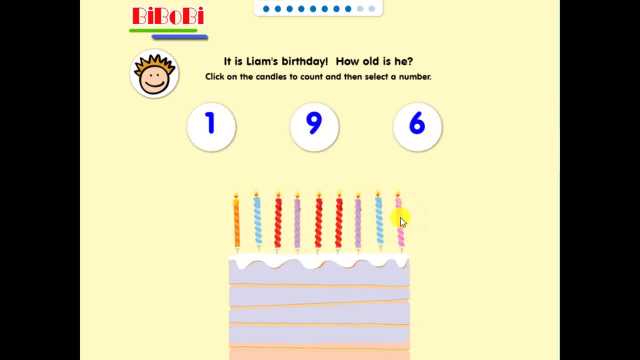 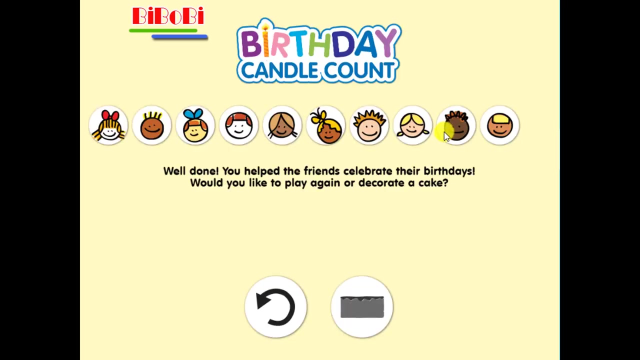 eight, nine, That's right. It is Susie's birthday. How old is she? One, two, three, four, five, Six, seven, That's right. Ava is a big girl. How old is she? One, two, three, four, five, six, seven, That's right. Well done, You helped the kids celebrate their birthdays. Let's decorate a cake for them. 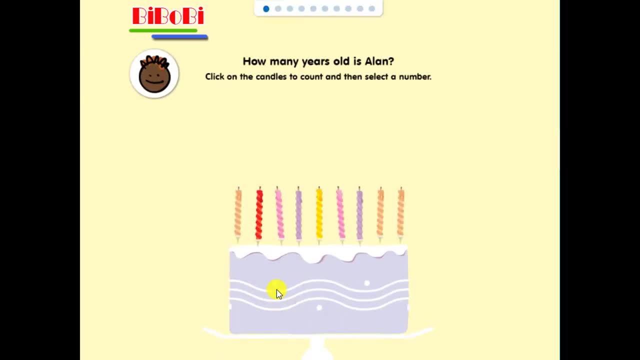 How many years old is Alan? Click on the candles to count and then select a number: One, two, three, four, five, six, seven, eight, nine, That's right. How old is Avery? One, two, three, four. 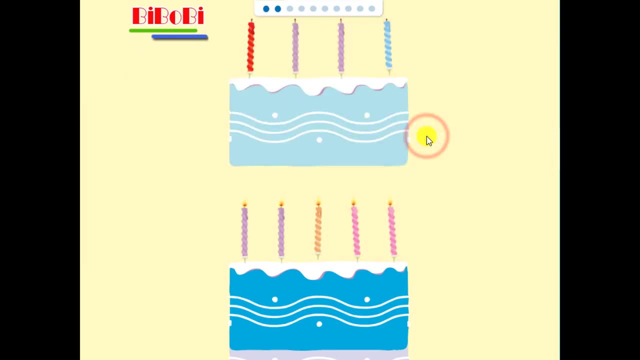 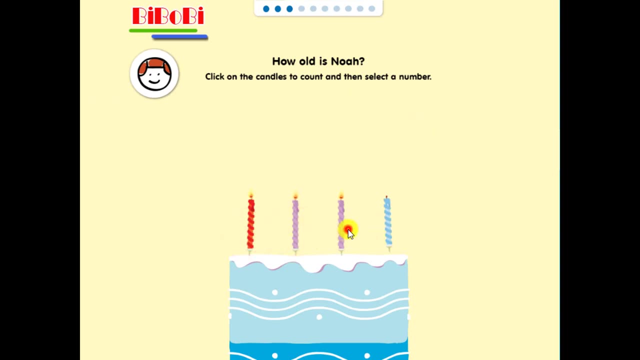 Six, seven, That's right, Ava is a big girl. How old is she? One, two, three, four, five, six, seven, eight, nine, That's right, Ava is a big girl. How old is Avery? 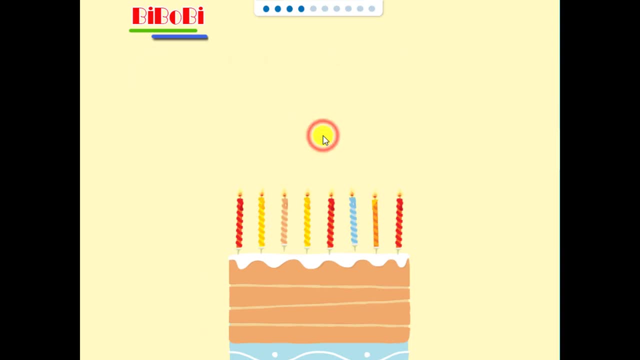 Eight, That's right. How many years old is Cormac? One, That's right. Busy is having a birthday party. How old is he? One, two, three, That's right. How many years old is Cormac? That's right. How many years old is Cormac? 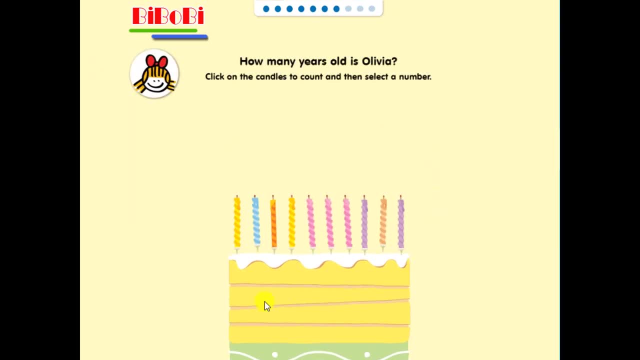 That's right. How many years old is Cormac? That's right. How many years old is Olivia? One, two, three, four, five, six, seven, eight, nine, ten, That's right. How old is Peyton? 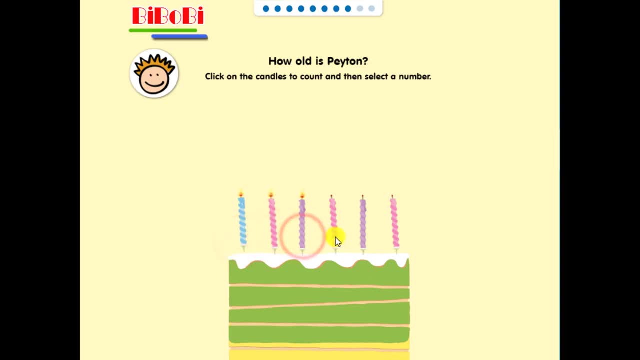 One, two, three, four, five, six, seven, eight, nine, ten, Six, That's right. Ian is a growing boy. How old is he? One, two, That's right. Tony is a big boy. How old is he?